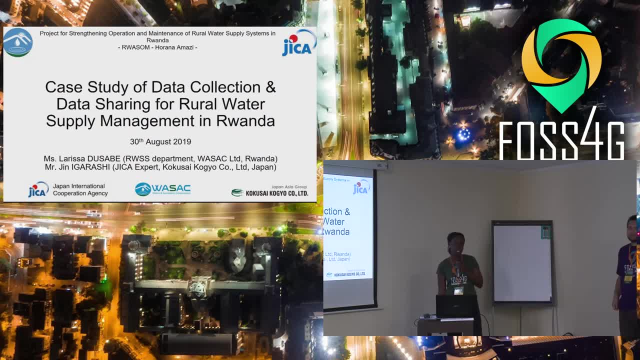 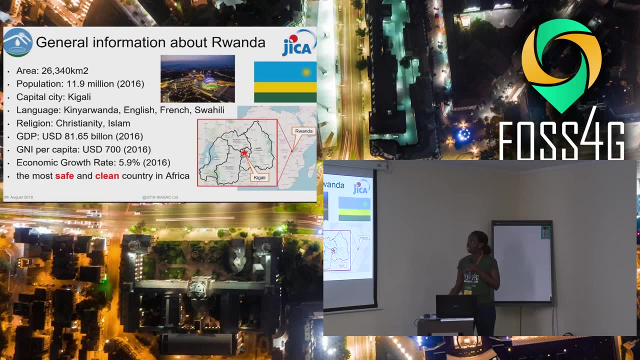 My name is Dusabe Larissa. I work in Wasak. It's a water and sanitation corporation that works in Rwanda- And my colleague is Gina Igarashi. he works in JICA. he's a JICA expert. We are currently having like a technical collaboration. 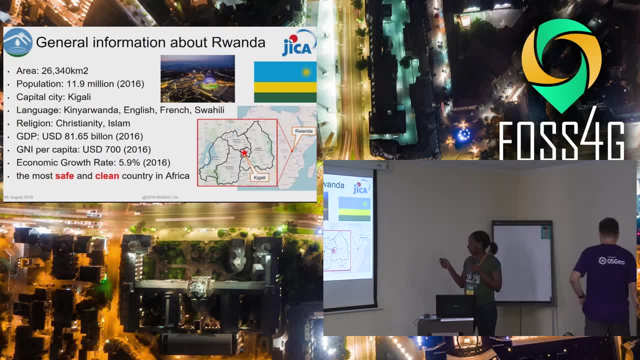 So Rwanda is a small country Located in East Africa and the capital city is Kigali. We have like 11.9 million population and our superficie is 26.34 kilometers- Thousand kilometers- And the language spoken are Kinyarwanda, English, French and Swahili. 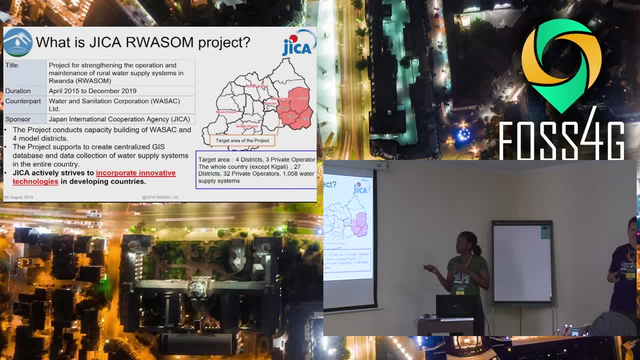 The original Islam and Christianity. So JICA: It has a project in Rwanda called Rugwasom. This project aims at strengthening the operation and maintenance of rural water supply systems. It started in 2015 in April and will end in December 2019.. 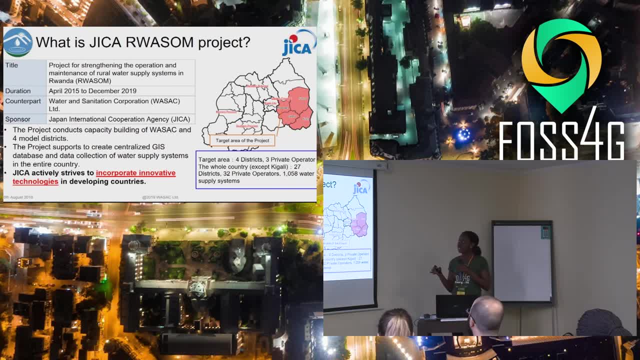 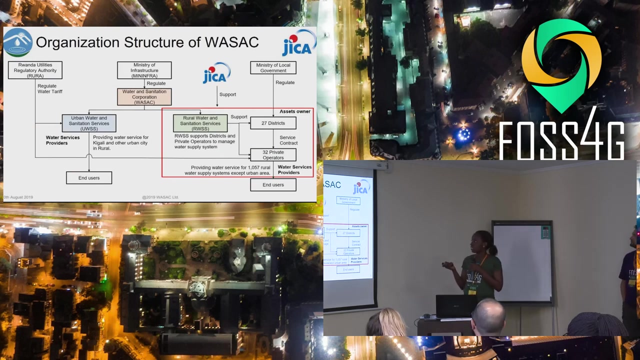 So we had the capacity building of Wasak staff and Fomodo district. They are the eastern districts. They are the one that endured several droughts Due to their locations. So Wasak has two main services: The urban water and sanitation services, where he is a service providers. 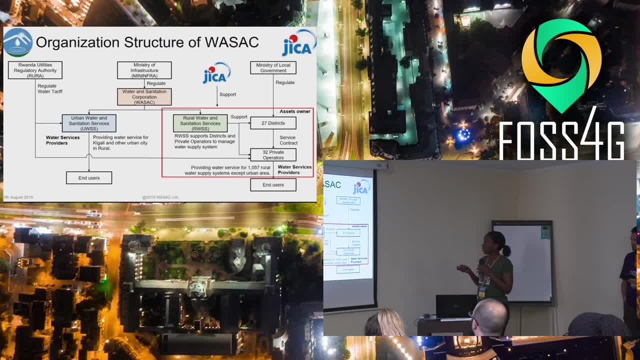 He supply water to the end users And in rural areas he acts like a supporter because the infrastructure are owned by the district. They are the one that are the infrastructure owners And they hire like private operators. We currently have 32 private operators in 27 districts. 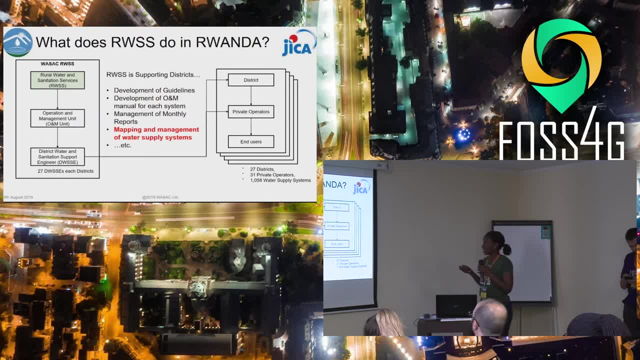 So what Wasak does the rural department? it develop guidelines And the operation and maintenance manual for each system, for the sustainability of the system, And we manage their monthly report to see if they are like working efficiently. They are providing good services. 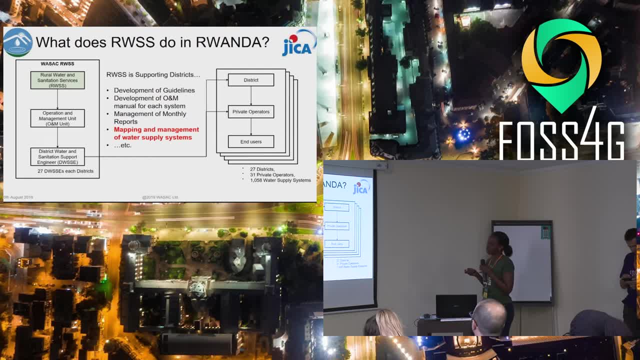 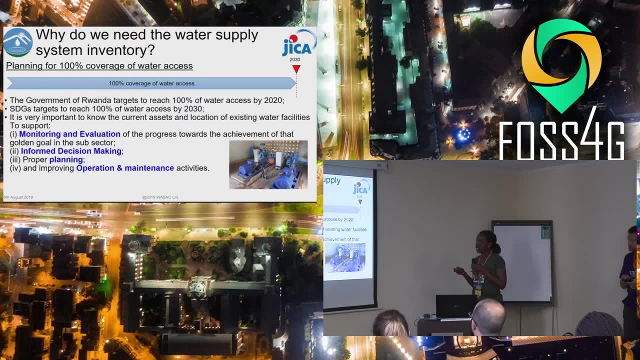 And currently we were working on mapping and management of water supply systems. So we targeted to reach 100% of water access by 2020.. And, as we know, SDGs targets 100% in 2030. But we couldn't achieve it without knowing the current assets we had. 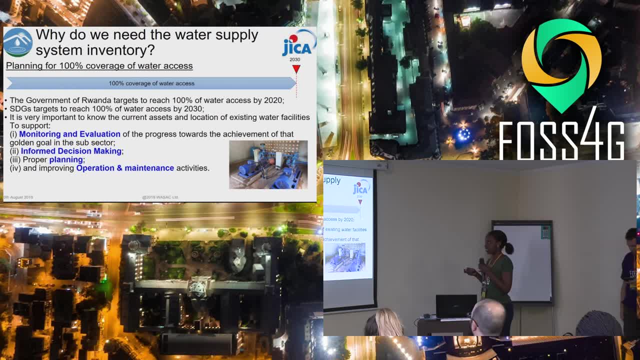 So that's when the data collection came in: For a better monitoring and evaluation Of the water supply system we had And to make proper decision. Like to know whether we need to improve our services or expand our network And in planning like new project, new water supply system project. 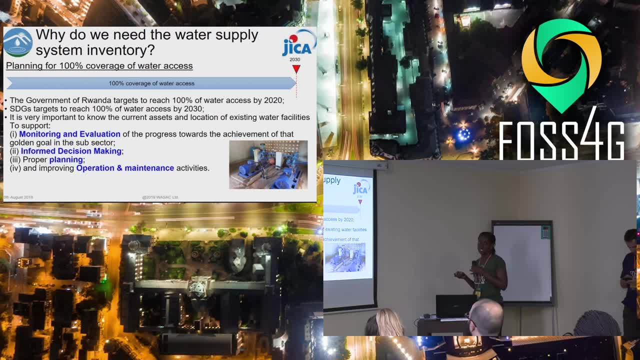 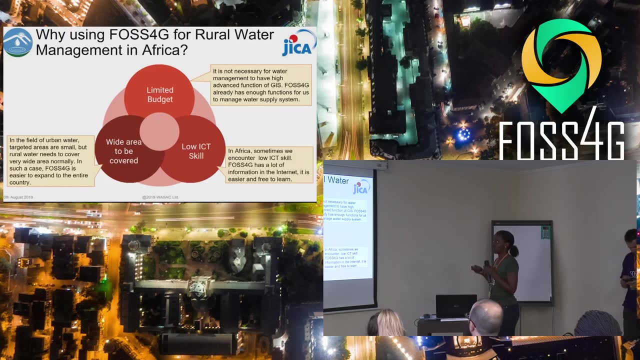 And also improving operation and maintenance activity. Like, if you don't do operation and maintenance activity in a good manner, Your system will not be sustainable. You will have to reinvest. So why using Phos4G? Because we had a limited budget. 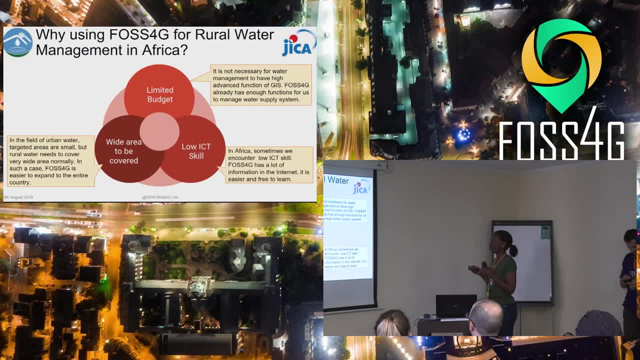 And it's easy with Phos4G. this problem was solved And we had a wide area In urban areas. the target area are currently in Rwanda. it's very small, So Phos4G is more easier to expand And for the skills also. 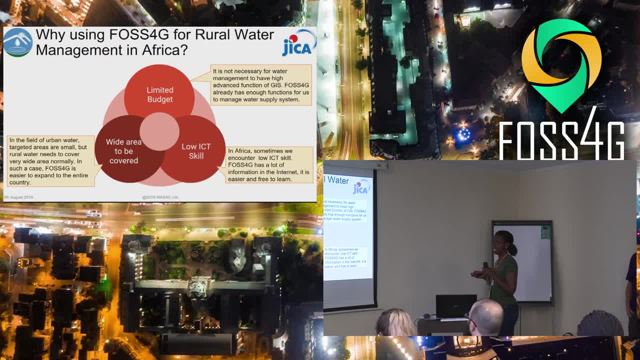 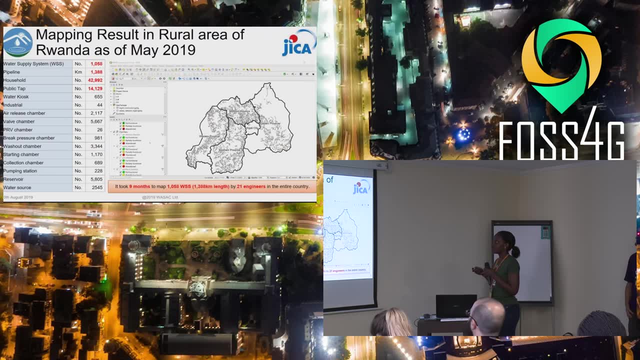 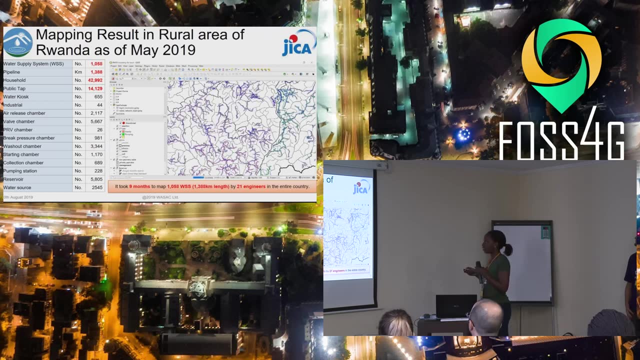 You can get more information on the internet for Phos4G So you can learn for yourself. So that's the assets. So that's the assets we collected. We went from each water supply system from the source. We featured all infrastructure components on each water supply system. 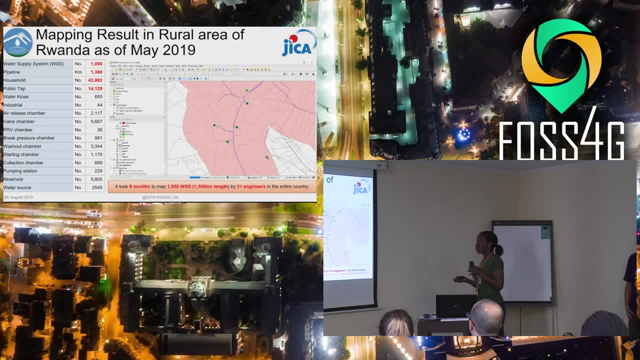 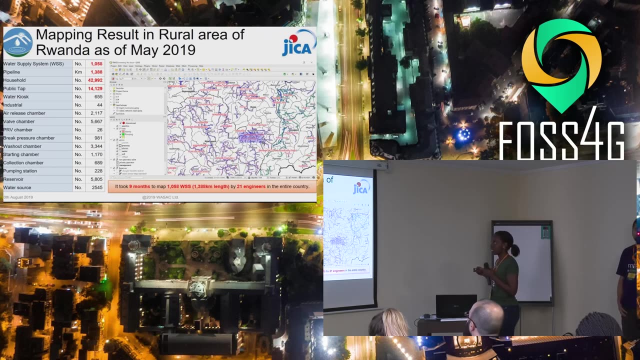 And their attributes, Like what they were built, Their equipment, Discharge, All those materials, etc. So we have- We currently have like 1.058 thousand water supply systems And the length of the pipeline are 1.388 thousand kilometer. 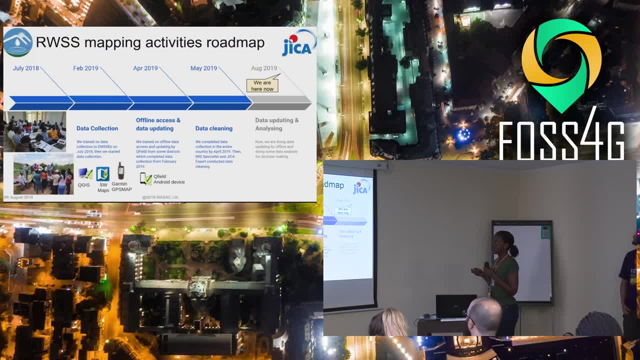 So this is the road map From July to February 2019.. We had a training on data collection Of district water and sanitation support engineer. They are the one who were in charge of correcting the data So that we can get accurate data. 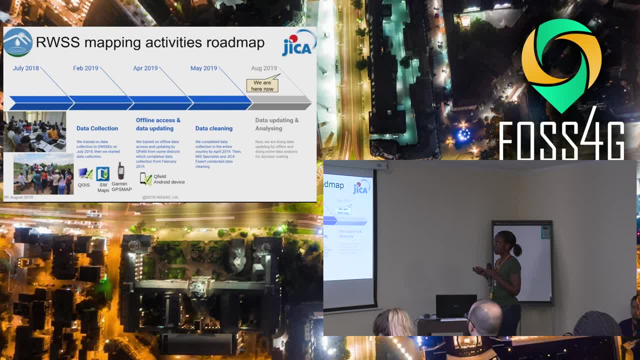 And from February 2019 to April 2019.. We had like, offline access Because we are working in remote areas. You can't rely on internet accessibility And you need, like You need to. You need to have data, Access to data for everyday operation and maintenance. 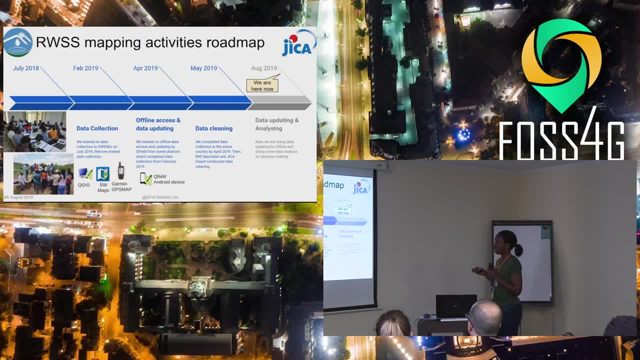 And from April- From April to May- There was data cleaning. It was done by MIS specialist And JICA expert To Like to have a database of Well and accurate data. So now we are on the stage of Data updating and analysis. 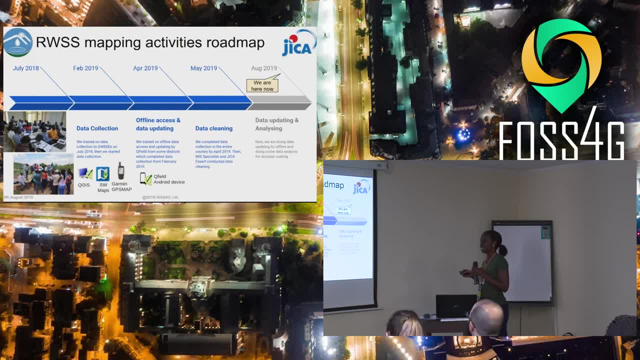 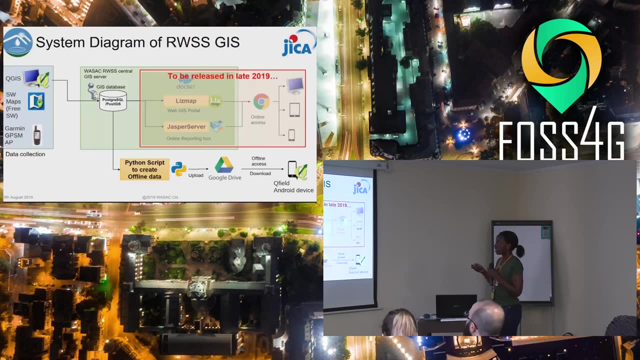 We make analysis on To select areas That are most That most need To have, project Water supply system project- So that we can work toward Achieving our target. So So, this is the Diagram showing all the process. 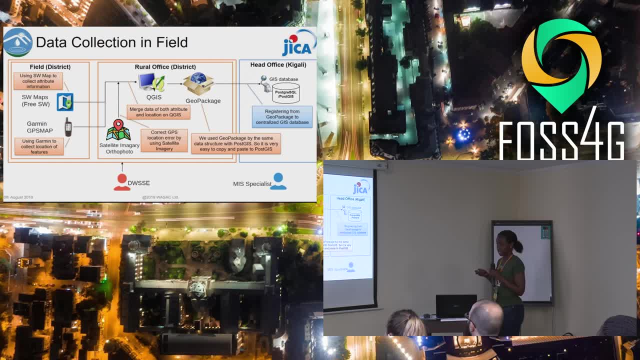 So for data collection We use GPS And SW map. It's not an open source, I know, but It's easier to record attributes Like information you need to fill in And to To correct the GPS location error. We use the. 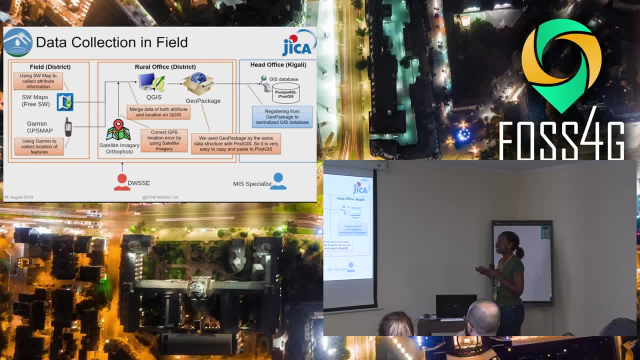 Satellite imagery Or to photo Or to photo, And then We match data and attribute And location And QGIS And we use the Geo package By the same data structure With post G's. So it's very. 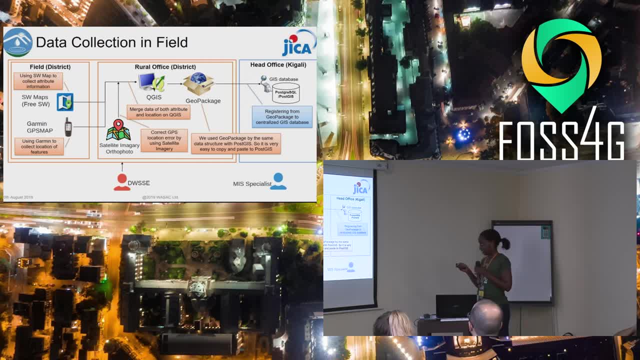 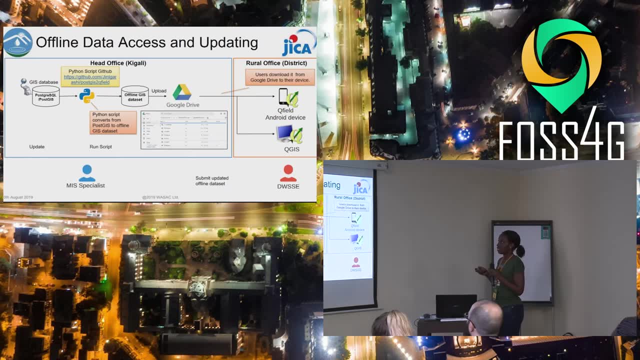 It was very easy to copy To the post G's. So for Offline data access We Run a script To take the GA, The post G's, To the Offline data set And then Upload it to. 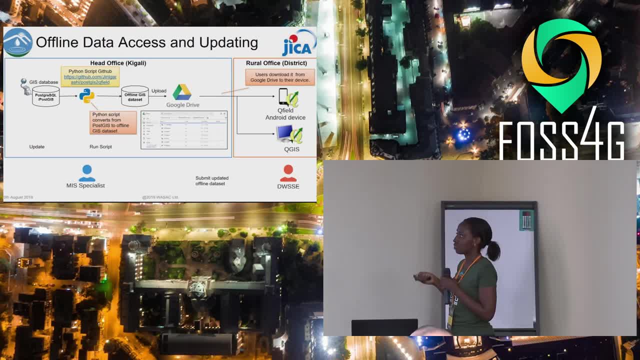 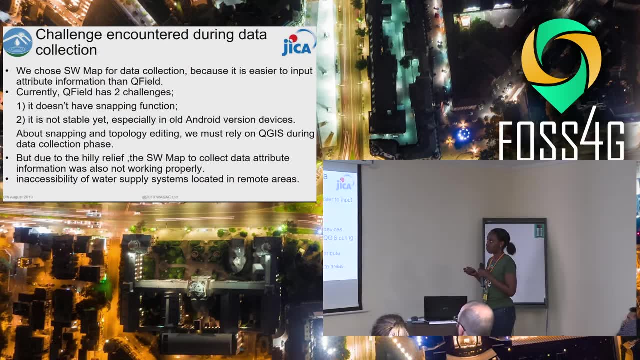 Google drive And the users Could download it Easily. So So The challenge We encountered During the Data collection Mainly Q field Doesn't have A snapping Function, So you can't Like. 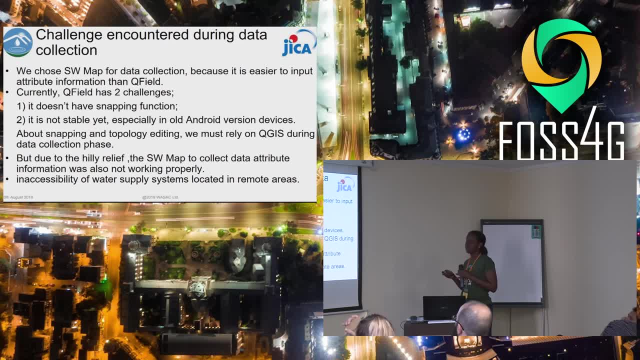 You can't, You can't, You can't Draw A network Without Having A snapping Option. It Couldn't Be Possible And it's Not Sable For Old Android. So. 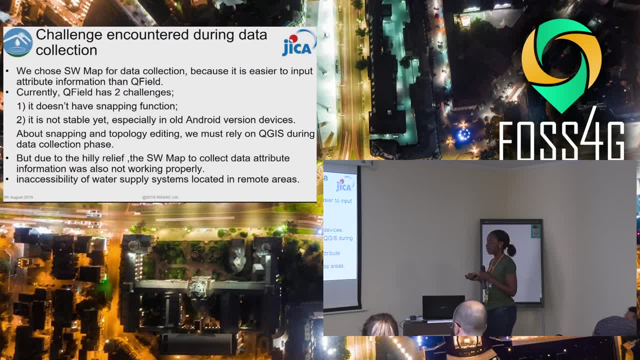 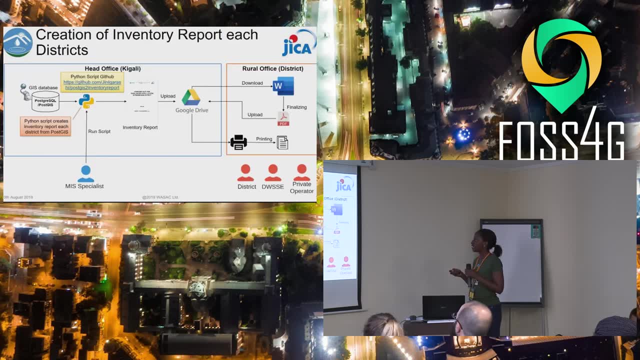 We Had To Adapt Ourselves And Some Water Supply System Were Located In Remote Areas. So We Plan To Have Like A Report That Could 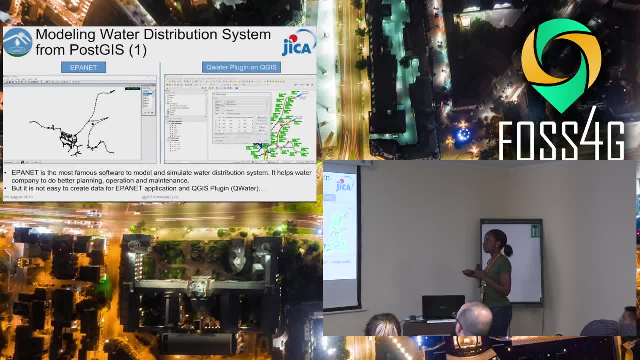 Be Produced Online By System. There Are Some Parameter That Need To Be Monitored, So That's When A Planet Is Needed, But It's Not. 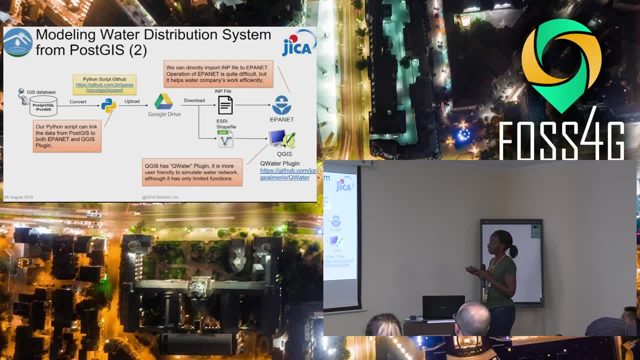 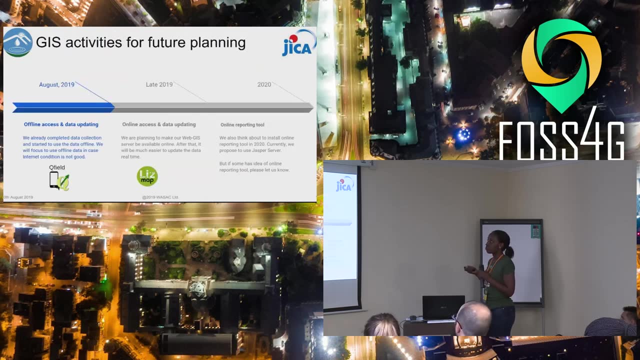 It Helps In Planning, Operation And Maintenance. But And See As She File Well Downloaded To A Planet And QGIS Where There Is Quota. 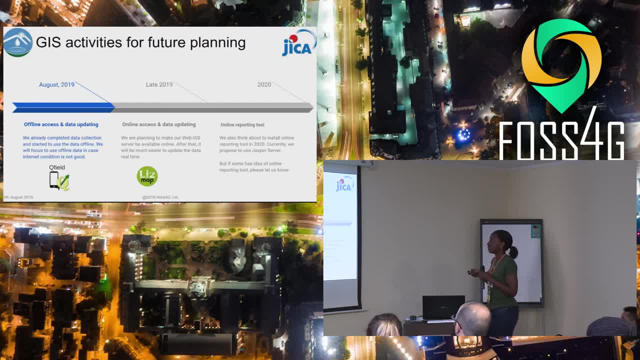 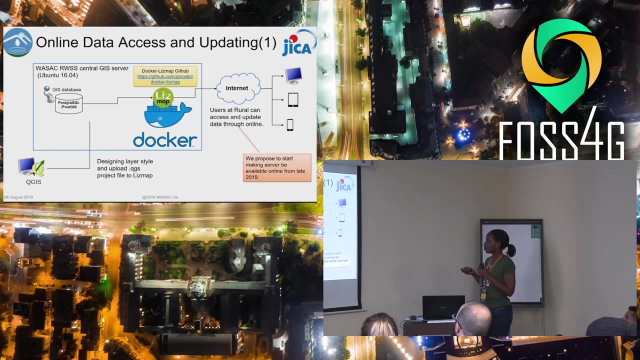 Plugin. So What We Are Planning In The Future. From Now On We Think In New Attribute Is Is More Easier Than Q Field Online. 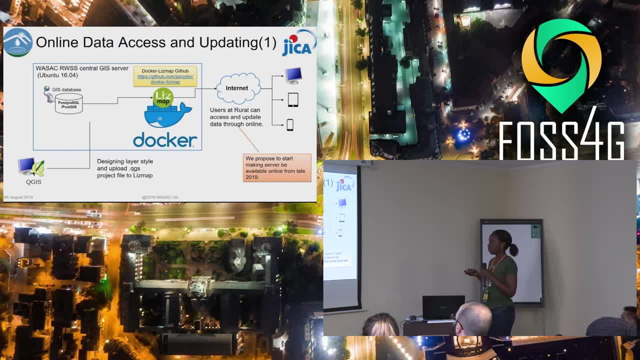 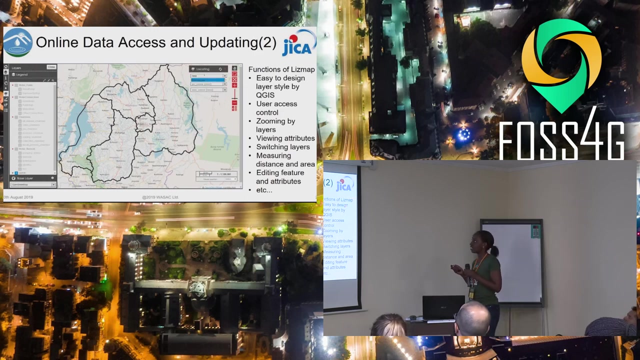 Reporting Using Just Per Server. So This Is How It Works. QGIS, We Design Layer Style And Our Devices. So Why This Map? Because It 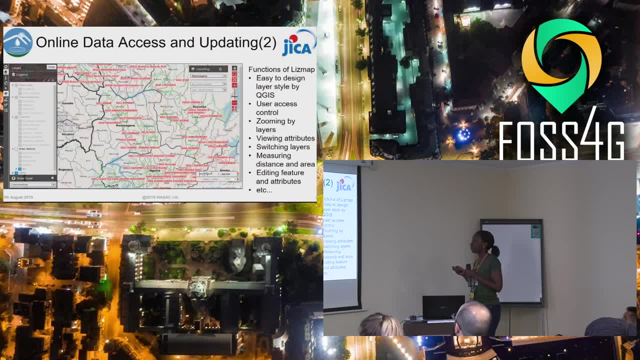 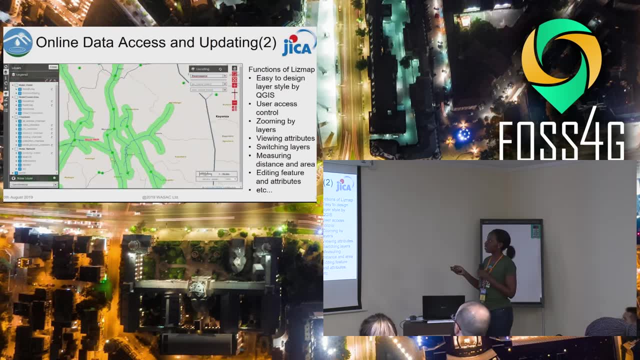 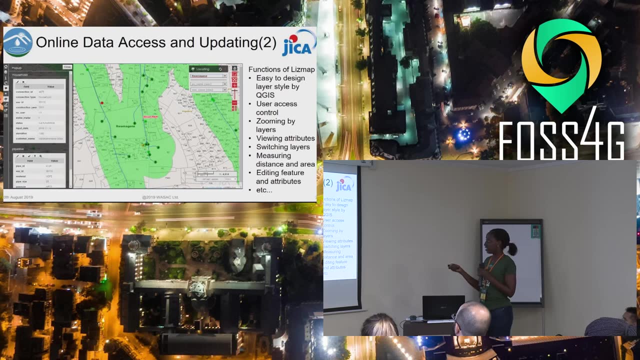 Is Easier To Design Layers In More. It's Easier To Design Layer Style By QGIS User Access Control And Zooming By Layers. And. 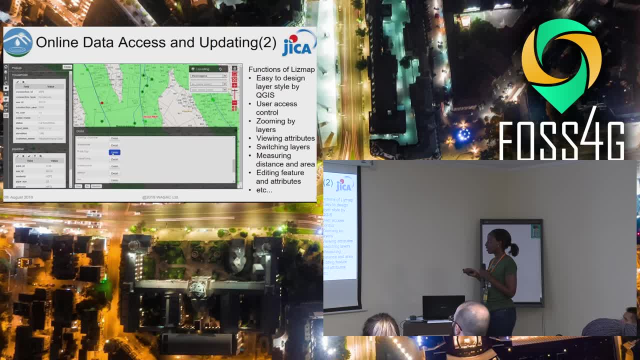 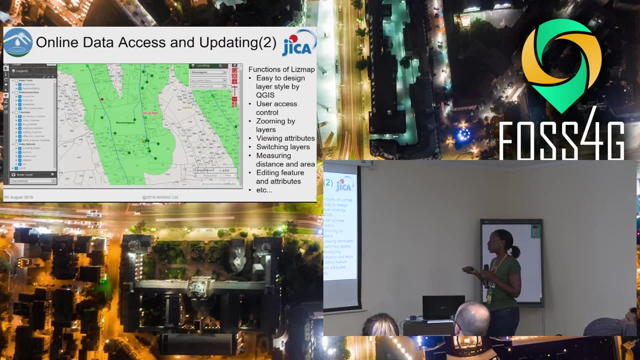 Viewing Attributes, It's More Easy Also- And Switching Layers Measuring The Distance And Area As You Can See It's, You Can Do It Like. 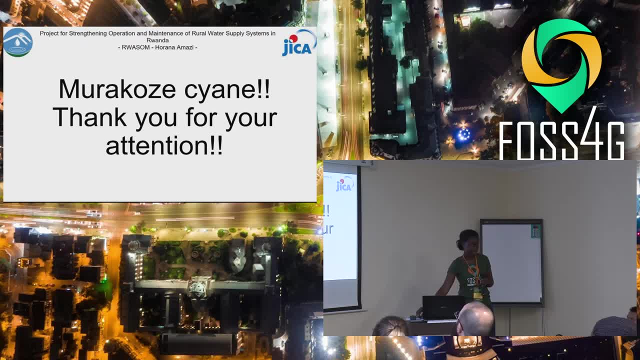 By Inserting The Researches. We Are A Little Bit Earlier Than Questions, But If You Have Any And Maybe We Have Enough Time For Questions- 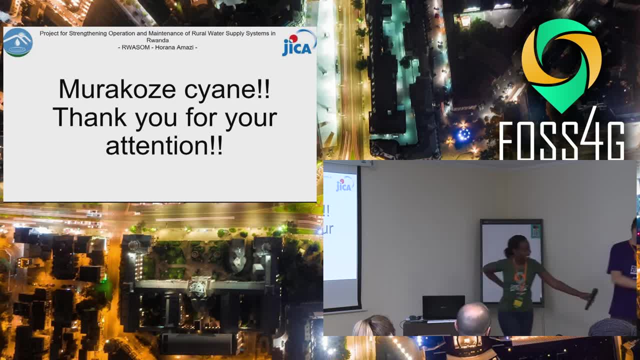 And Answers. So Just Please Start Away. Did Any Versions Or Just The Old Ones? But The New Ones Work, The Old Ones Don't Did. 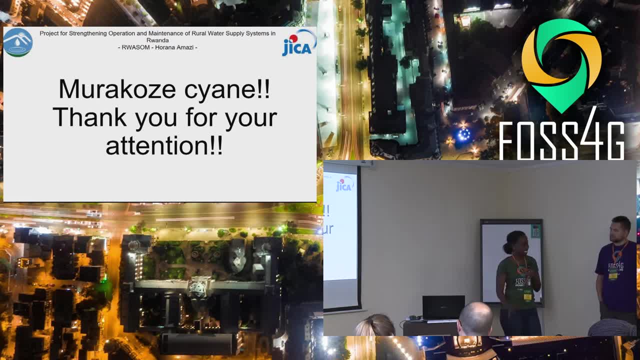 You Test This Financial Issues. So Many Of Our Users Don't Have Any Questions About The Procedure. If I Understood Correctly The Actual, Let's. 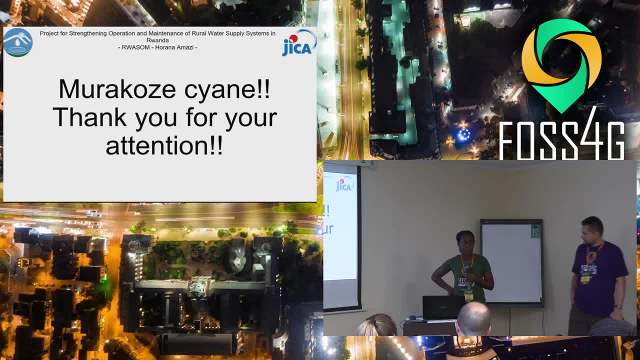 Say, Data Collection Was Done By A Group Of Engineers Which Went On The Ground And Is. We Are Now Starting To Train Local Person, Local 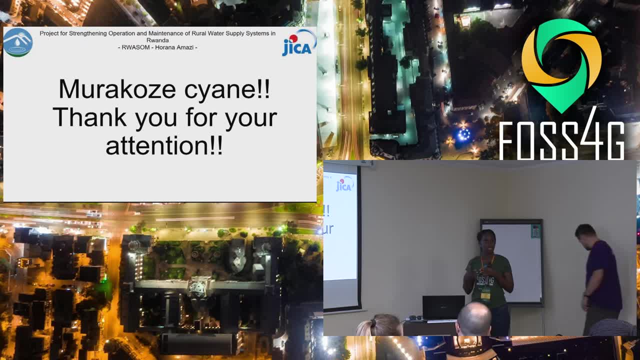 Technician How To Do It So That The Engineer Don't Have To Go Back To Decide To Get The Data. So I'm Going To Share. 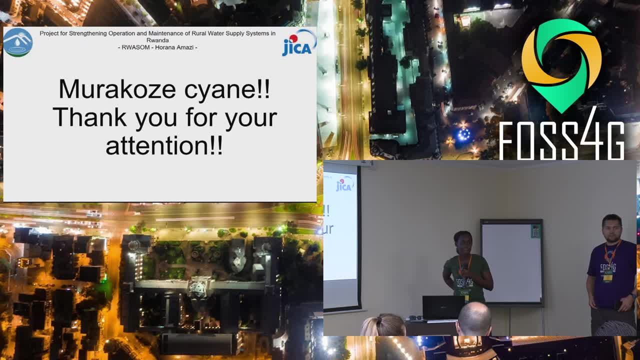 This Also With My Colleagues From Fitness Avidus International. We've Worked On This. This Is One Question From My Experience In Rwanda: How 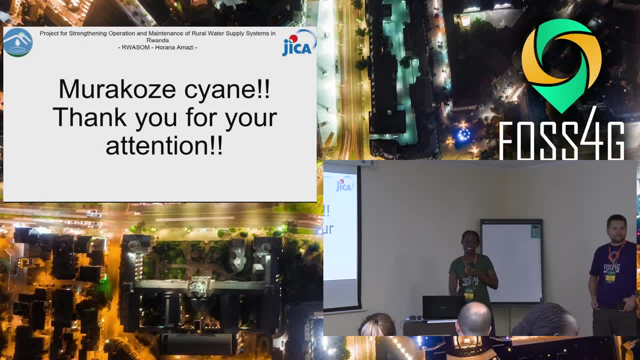 Easy. As You Remember From What We Discussed Before That, When We Wanted To Do A Project With QGIS There, That All The Donors